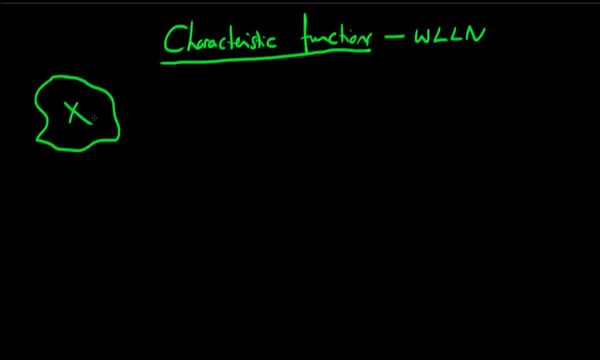 of their probability distribution. Can I prove it just in terms of the properties of that random variable x as it stands? Well, sometimes that's not possible, But I can transform my random variable to a new space, which I'm going to call characteristic function space. 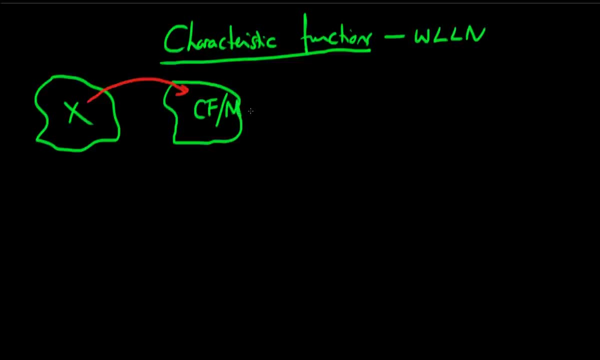 or another sort of transform you can think about is something which is called the moment generating function, And then if I can prove something about my random variable in this space, then it turns out that this holds when I sort of transform back to my random variable. So I would have. 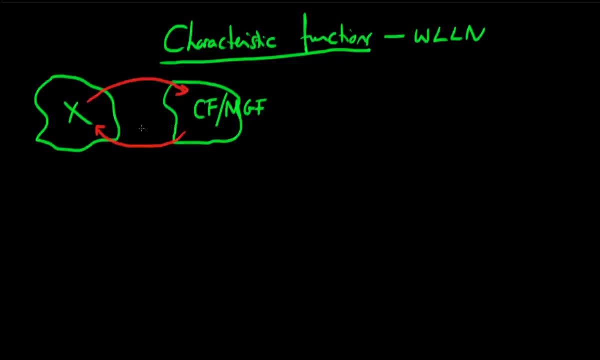 actually proved that sort of thing that I was trying to prove about my original random variable. So why can we do this? Well, the idea is that for every different random variable- say whether it be Poisson, normal, binomial- each type of random variable has a different 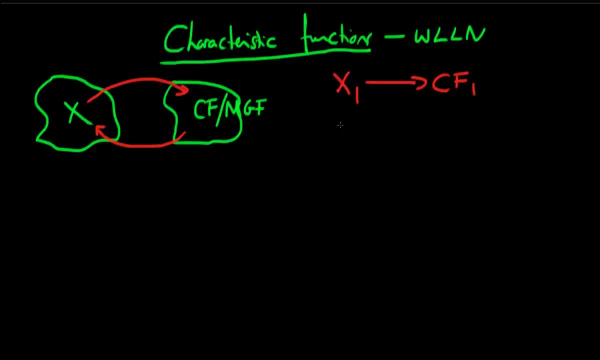 characteristic function. So if we sort of think about an example: random variable x1, that has a characteristic function cf1.. Variable two has a characteristic function cf2.. Yeah, and you can sort of think about this for every different type of random variable. 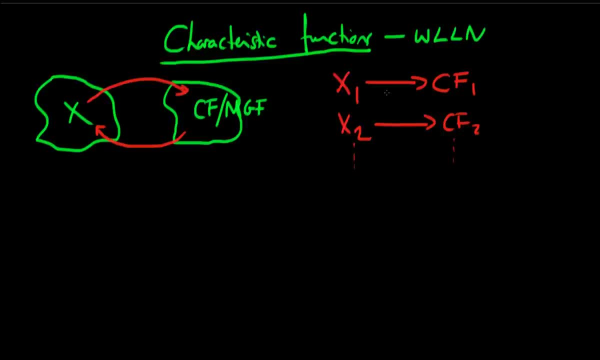 there is an associated characteristic function. So it's just sort of one to one mapping, But this mapping also holds going the reverse way. So for every particular random variable, every particular type of characteristic function, there is only one type of random variable with an associated probability density that can satisfy that particular characteristic. 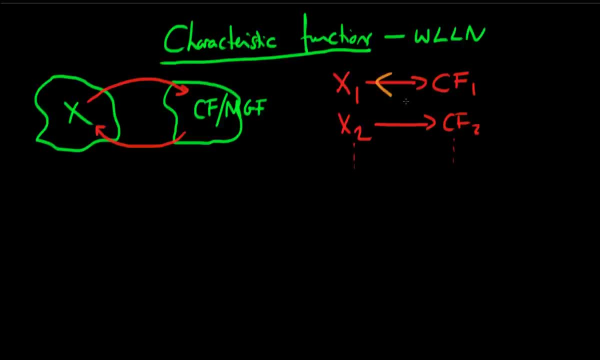 function. So this property is a very nice property for characteristic functions to have, because if we can show that, let's say, variables x1 and x2 have the same characteristic function, then they must represent the same underlying random variable, because there's only one characteristic. 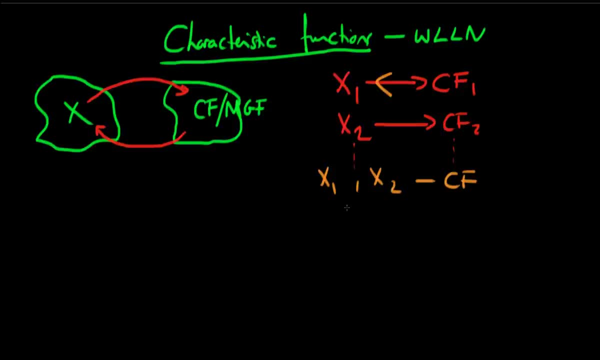 function Per random variable and vice versa. So that's why we sort of deal with characteristic functions. they're quite a nice property for them to have And it allows us to prove some theorems which we wouldn't be able to prove without their use actually. So what does it actually? 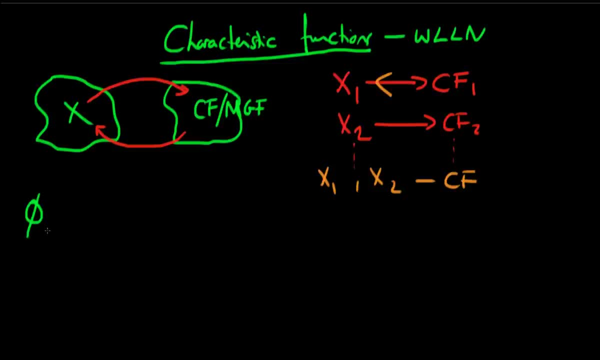 mean to find the characteristic function. Well, the characteristic function of random variable x is defined in terms of some parameters: t, which is part of the transform, And it's defined as being equal to the expectation function of the random variable x, which is 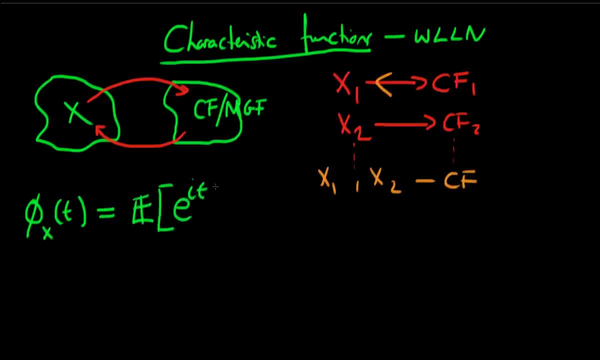 the expectation of e to the i t x. And well, what does that mean? Well, we just use the law of the unconscious statistician, which is we integrate from minus infinity to plus infinity, e to the i t x times our probability density. Yeah, So that's how we sort of calculate. 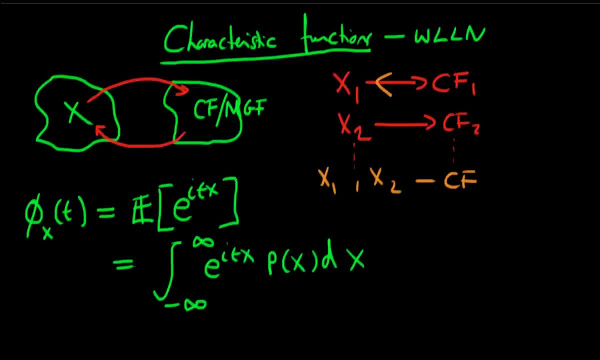 our characteristic function And in general this isn't necessarily that easier thing to do, because really what we should be using here is the characteristic function of random variables x, And what we're using here, because it's a sort of complex integral, is we should. 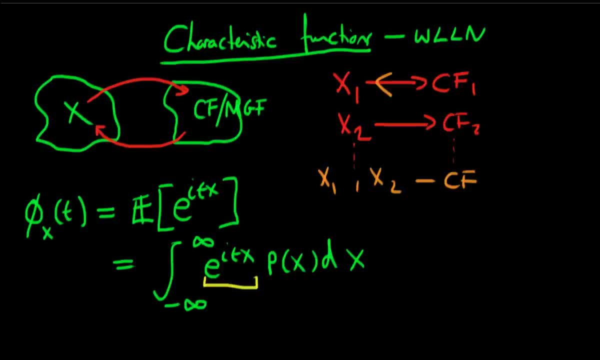 be doing some sort of complex analysis which, in sort of principle, isn't necessarily that hard to do. but it assumes that you know about complex analysis. Well, what are some of the properties which characteristic functions have? Well, one of the nice properties is: 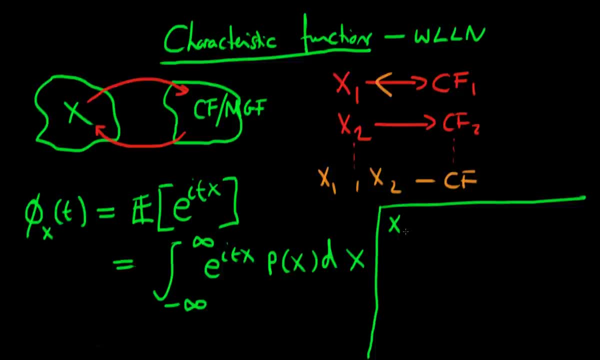 that if I have a whole host of independent random variables, x1 through, let's say, xp, so that's the characteristic function of x1 through xp as a sort of group, as a function of t. Well, that's just equal to, in the case of independent random variables, the product. 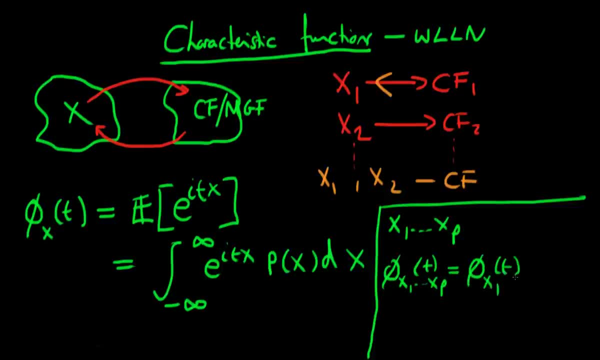 of the individual characteristic function. So that's phi of x1 times phi of x2 as a function of t sort of times all the way through to phi of xp as a function of this parameter at t. So that's quite a nice property for characteristic functions to have. If I have. 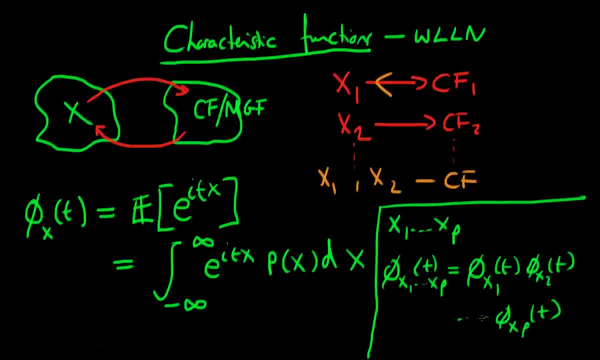 independent random variables, then the characteristic function of that group of random variables is just equal to the characteristic function of each random variable on its own multiplied by the other ones. So that's a nice property for it to have. Another nice property which characteristic functions have is that phi of some constant a times that random variable x. in terms of this, 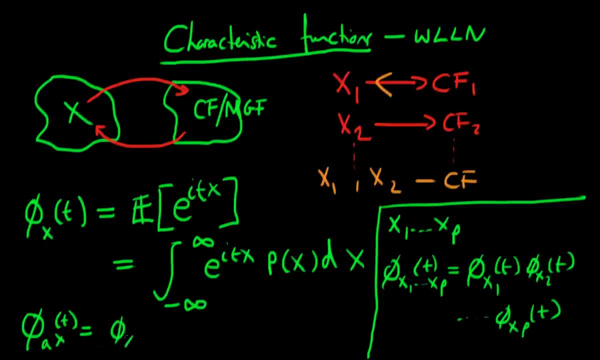 parameter t is just the same as phi of x as a function of a times t. And that's quite easy to see, because if I sort of multiply x by a, then it sort of just comes up here in terms of I get sort of e to the i, t, a, x.